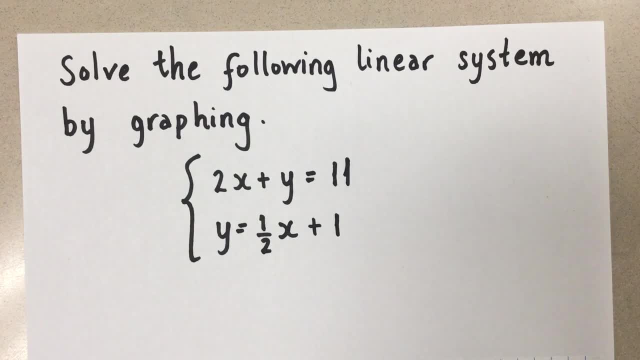 I have several videos on how to do this algebraically. So again, if we're solving a linear system, we're looking for the point of intersection between these two lines. If the two lines happen to be parallel, then they would not have a point of intersection, and if the two lines 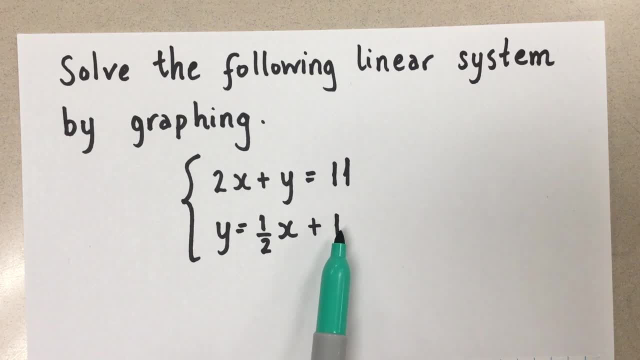 happen to be the same line, then we would have an infinite number of points of intersection, And in this case we are just going to have one point of intersection, and that is the solution to the linear system. So let's look at the two equations that we have. We're going to first work with the first equation here. 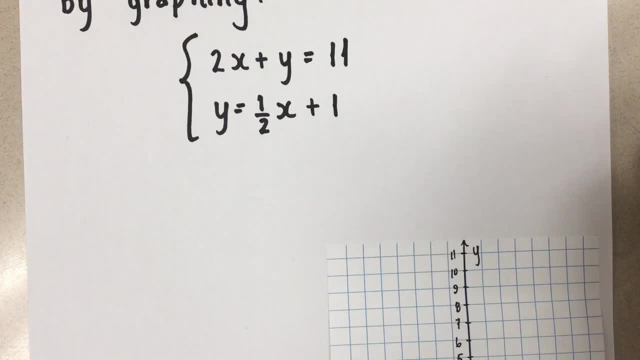 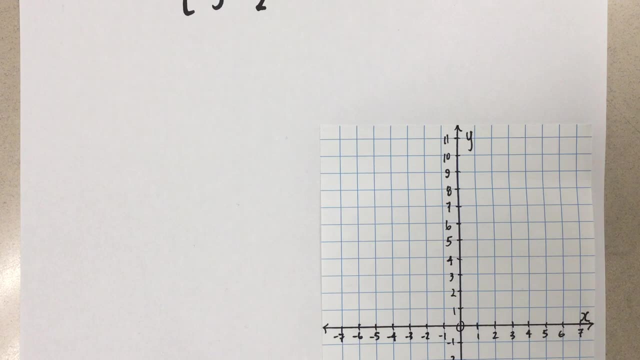 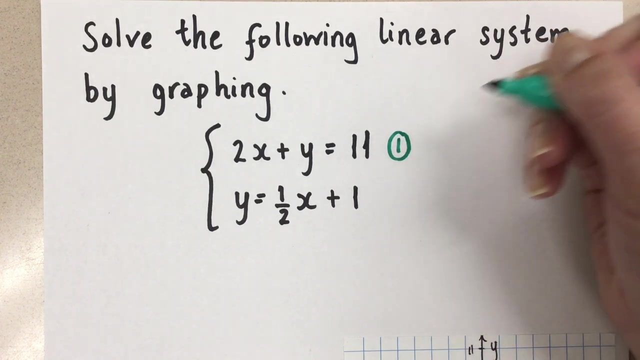 2x plus y equals 11, and I have my graph set up below here on graph paper and my axes are already labeled and the scales are done. I'm just counting by one on my scale today, So I'm going to look at this first one first. We can call this equation 1, if you prefer. 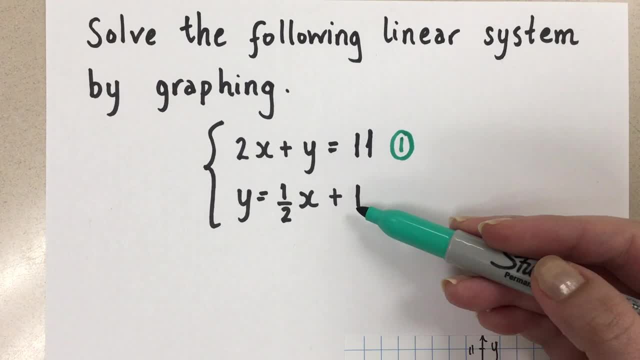 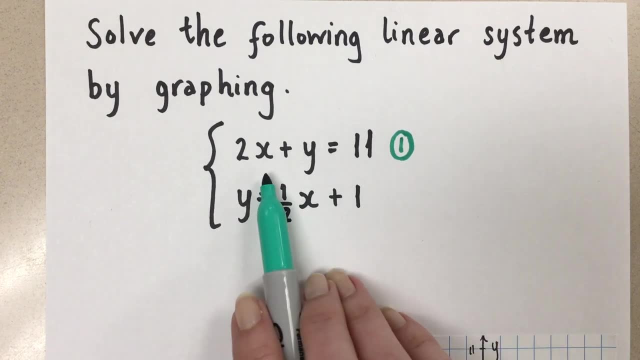 I'm going to use this teal color, and then we'll move to the second equation afterward. So the first thing I notice about this equation is that it's in standard form. The x and the y terms are on the same side of the equal sign. 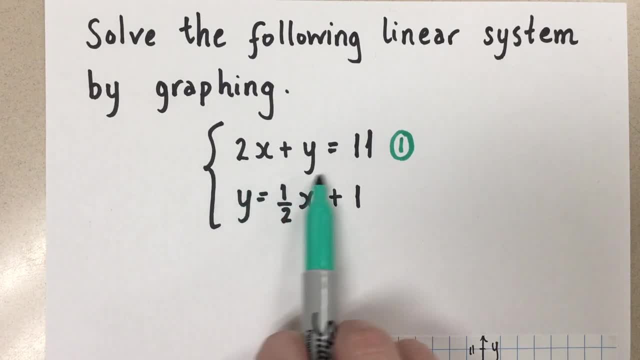 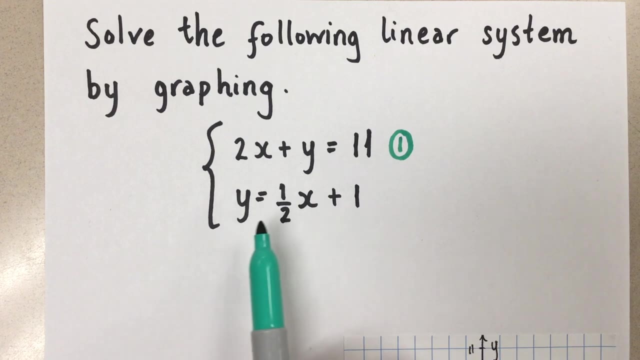 So the easiest method to graph this equation, based on the form that it's in, is to find the x and y intercepts. That will be the quickest way to do this. If you prefer to graph using slope y-intercept form, like our second equation is, then you can wait until we do the second one here. 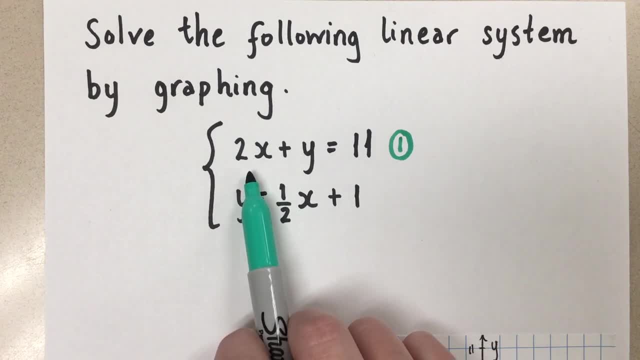 and I'll show you that. Or you can go and look at my video on how to switch from standard form to slope y-intercept form, and then you can do it that way if you prefer. But today I'm going to use x and y intercepts. 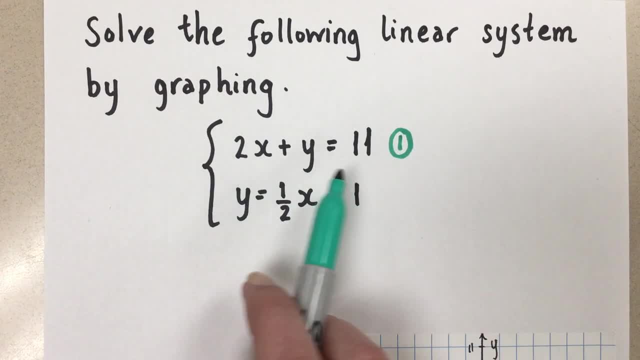 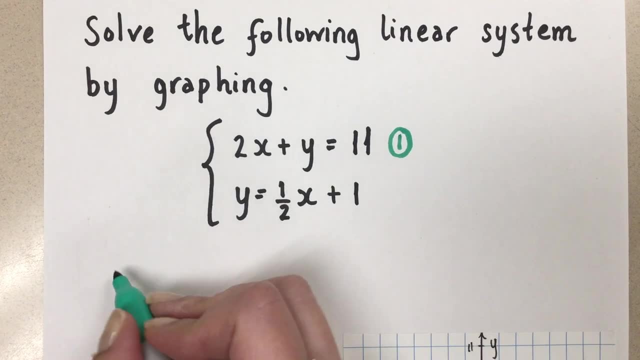 So if I want to find the x and y intercept for this equation, we're going to use the fact that when we have an x intercept, that point has a y-coordinate that's equal to zero, And so if I make use of that, then I can take that first equation. 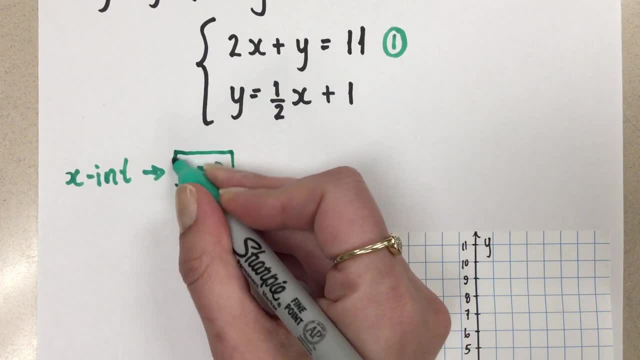 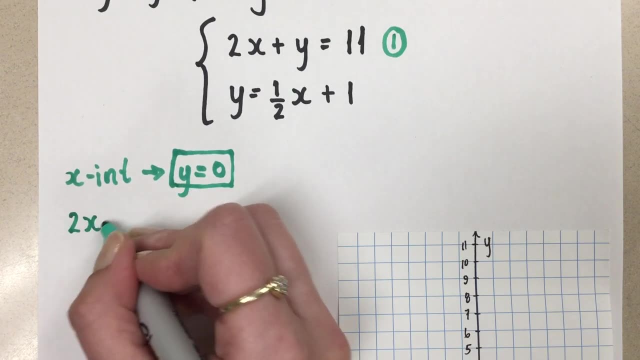 and sub in y equals zero and solve for the x-coordinate that matches the y-coordinate of zero. So my equation is 2x plus y Instead of y. I'll put that zero there. It's like we're subbing it in. 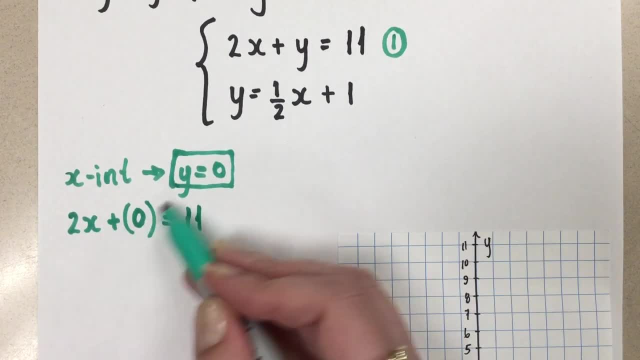 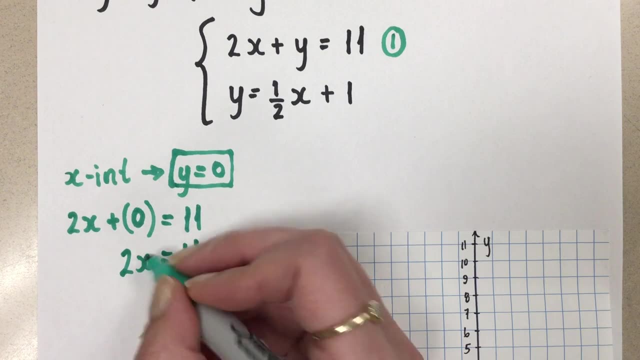 Equals 11x, And so we just have a plus zero there. We can eliminate that And we're left with 2x equals 11.. So here, when we solve for x, we can divide both sides by 2, and x is 11 over 2.. 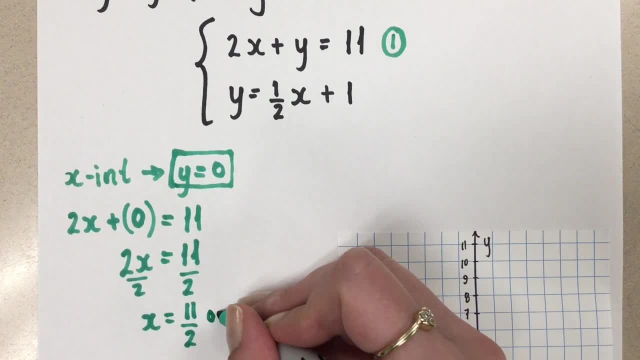 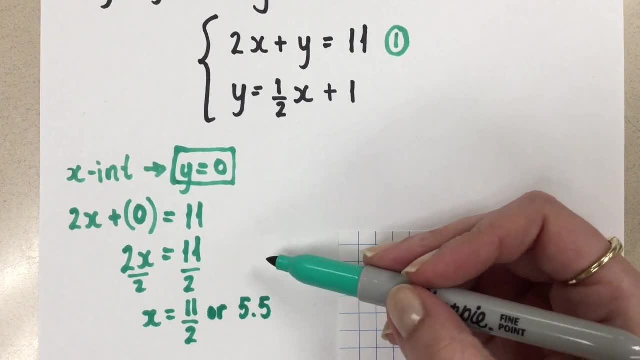 That's in reduced form Or because we're going to graph this. we can change it to a decimal. It might be easier to put on that number line And we get 5.5.. So this means on our graph here: 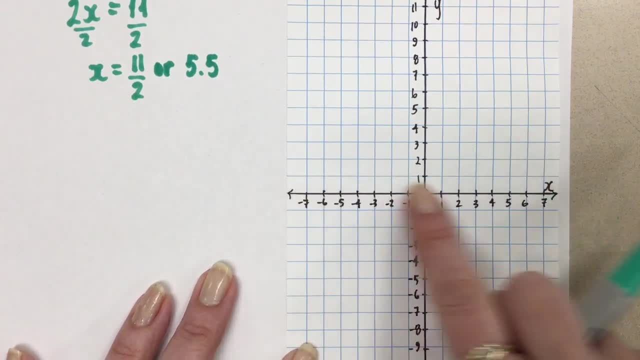 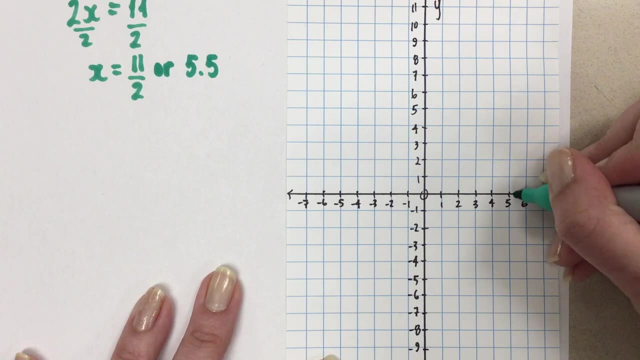 this line is going to be the y-coordinate of zero. This line is going to have an x-intercept, So on the x-axis it will cross at the point where x is 5.5.. And of course y equals zero at that point. So I'm going to plot that point there. 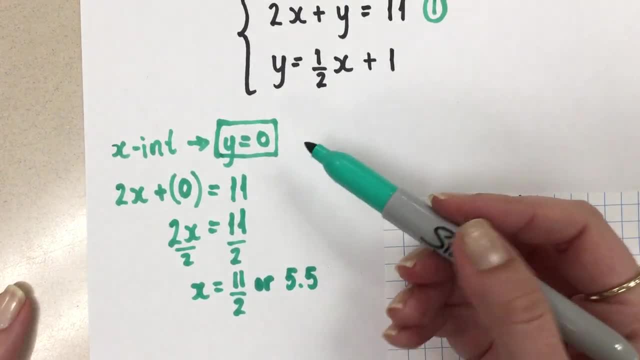 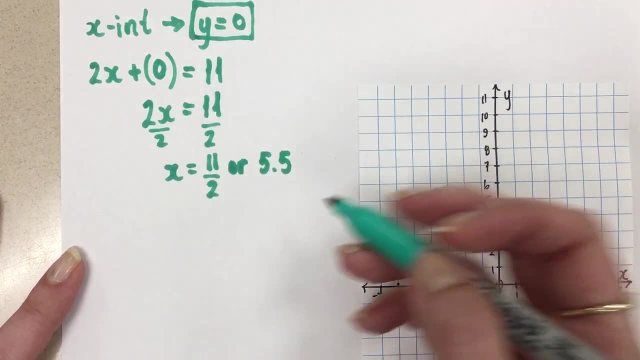 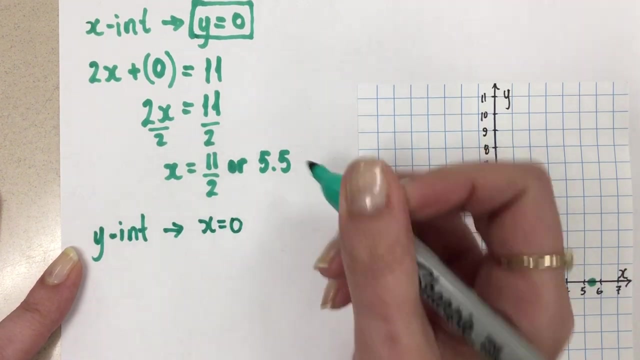 Okay, let's go ahead and do the same thing for the y-intercept of this line. So now, in the opposite way, if the x-intercept has a y-coordinate of zero, then the y-intercept has an x-coordinate. So I'm going to take that original equation of the line. 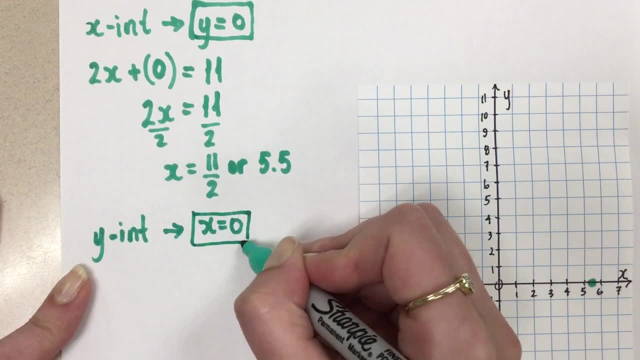 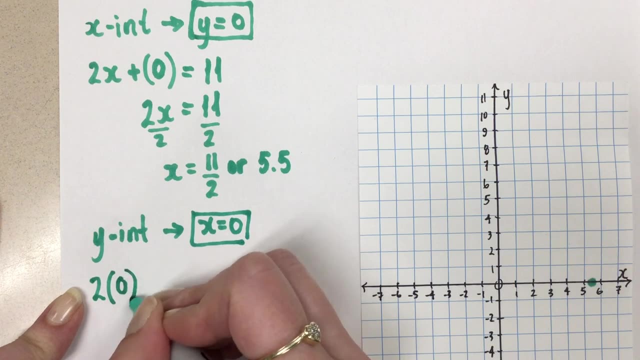 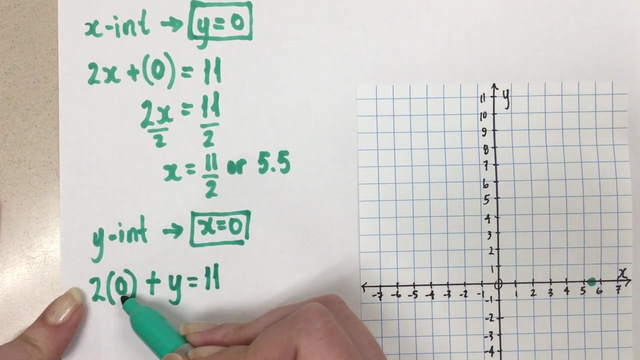 and I'm going to sub in zero for x and then solve for the corresponding y-value. So it'll look like this: 2 times zero, because that's where the x was plus y equals 11.. Okay, so now 2 times zero. well, that's going to eliminate. 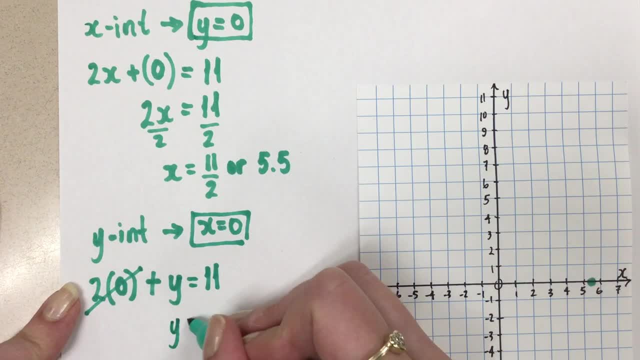 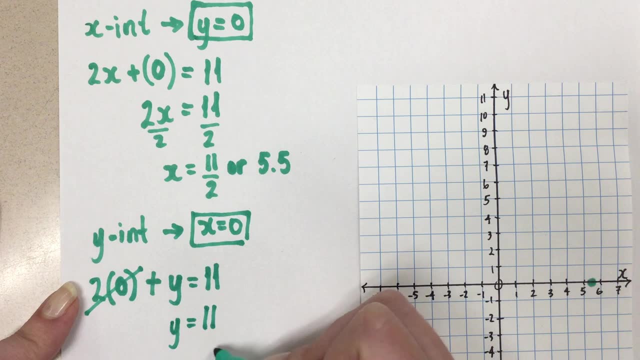 because that's just zero. And here we're left with y equals 11.. We don't have a coefficient, or I should say the coefficient on y is 1, so we don't need to divide by anything here. We just have y equals 11 as our y-intercept. 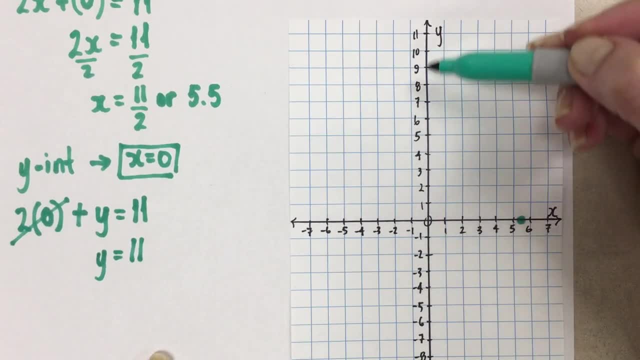 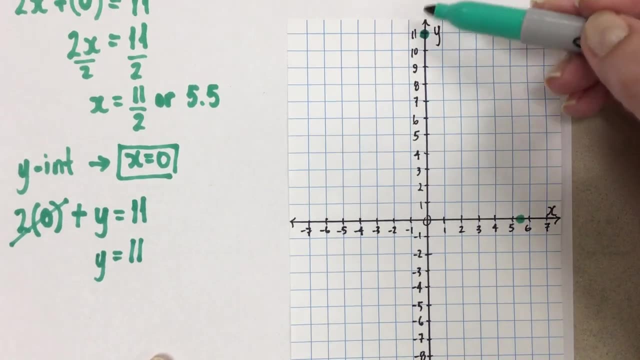 So we're going to go to our graph and on that y-axis I'm going to plot a point at positive 11, and of course the x-coordinate is zero there. And so now my y-intercept here and my x-intercept here. 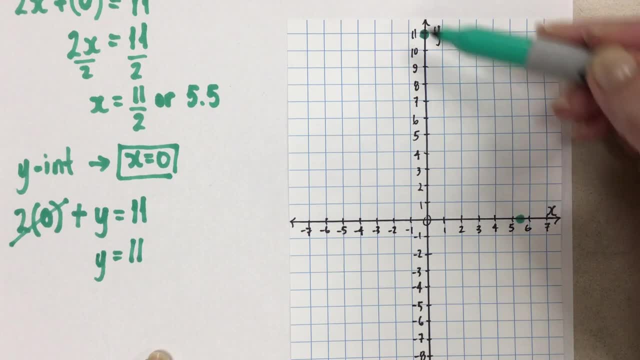 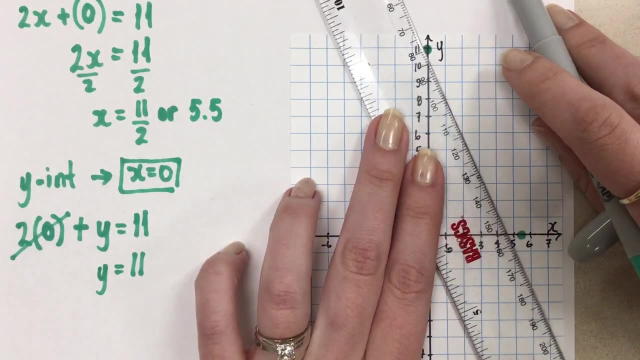 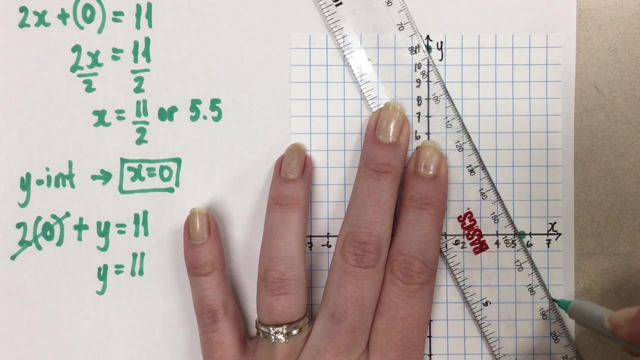 show where that line is going to cross, because any line only requires two points to draw, So I'm going to draw that line between it. So I'm going to go ahead and do that Here very as accurately as possible When we're doing our graphs for solving systems of equations. 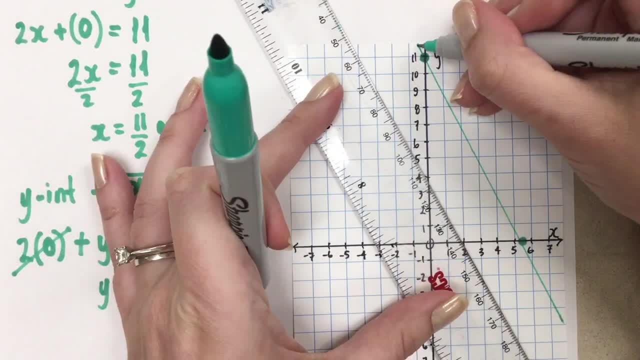 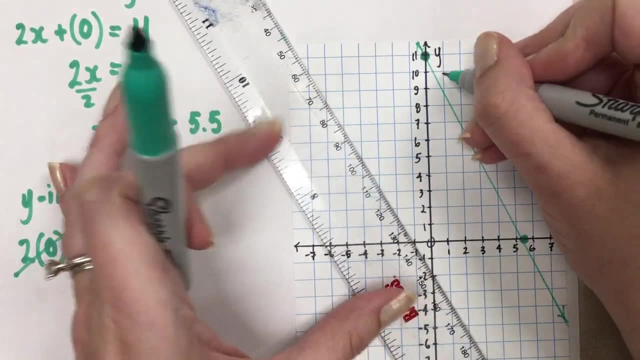 we really want to try to be as accurate as possible. There is always a little bit of human error, but it's necessary to be as accurate as we can here. And I'm going to label that line with the equation because we want good communication in our math. 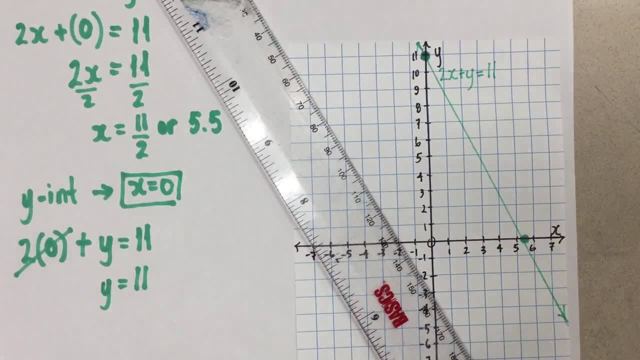 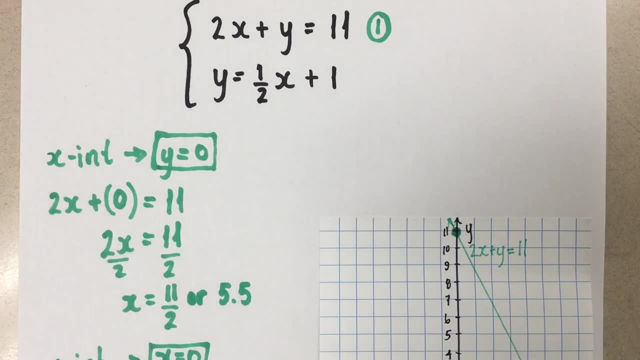 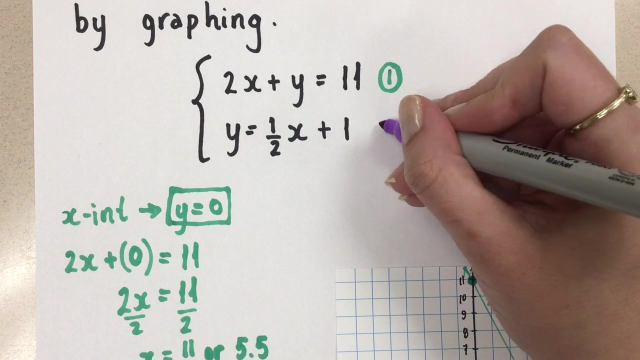 2x plus y equals 11.. So here's our first line that we drew. Now let's go over to the second line. Here we have y equals 1 over 2x plus 1.. Let's call this line number 2.. 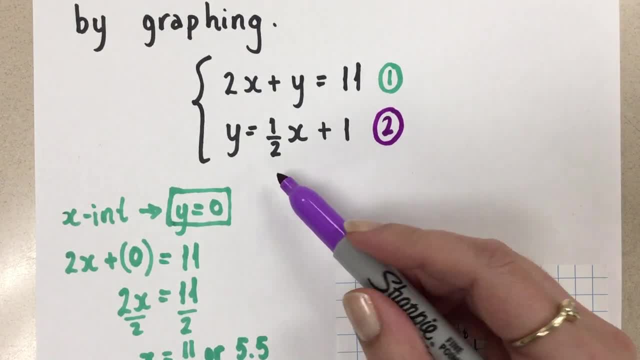 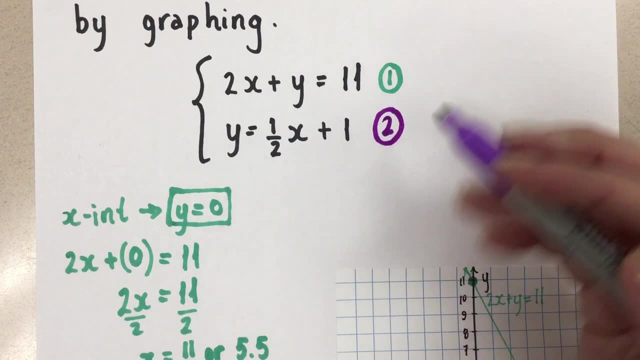 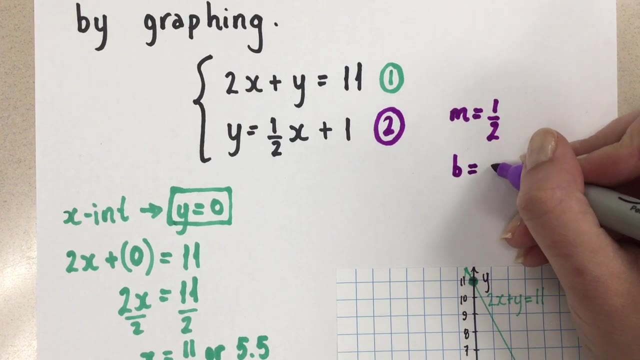 And we're going to graph this one using its slope and y-intercept, because this equation is in that y equals mx plus b form. So here our slope and y-intercept. Our slope is 1 over 2.. And our y-intercept is positive 1.. 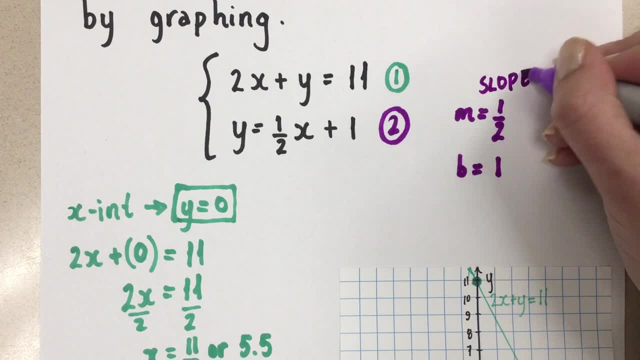 If our slope here- so this is our slope, let's label it is 1 over 2, then we know that that 1 represents the rise and that 2 represents the run. So here we're going to go: up 1 and to the right, 2. 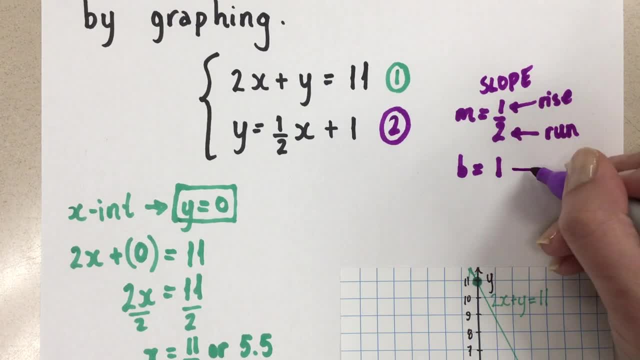 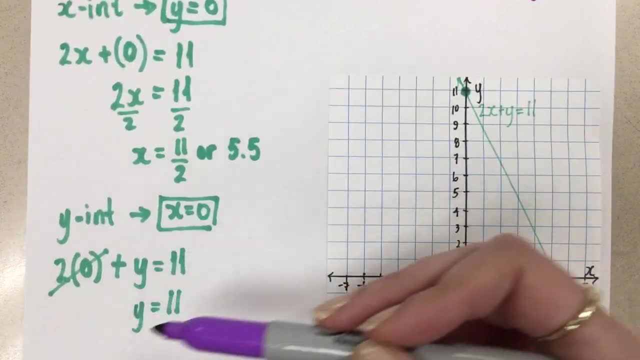 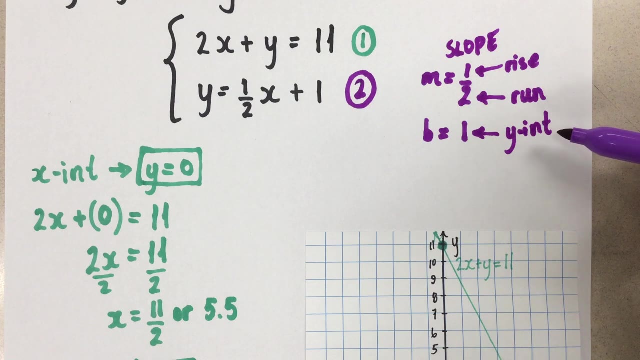 as we move across our line. This is our y-intercept. So we're going to use this y-intercept in the same way that we used it when we found the y-intercept for this equation. here We're going to go to our graph and start graphing this line on the y-intercept. 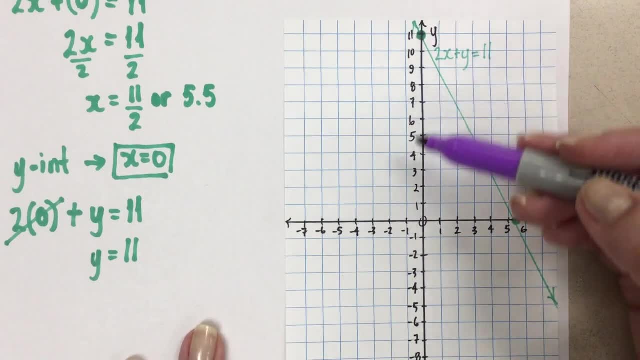 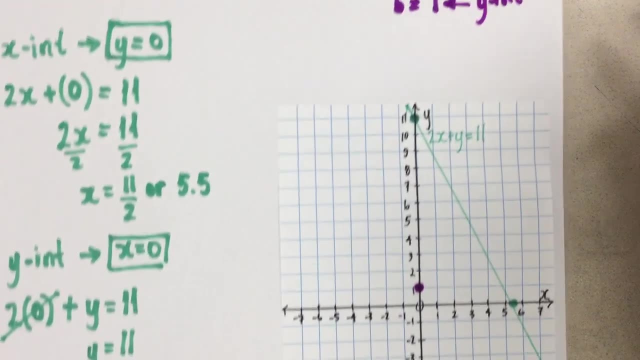 So a y-intercept of 1 means that on this graph on the y-axis, we're going to plot our starting point at positive 1.. And then we're going to use the slope from that point, we're going to go up 1 and we're going to go right 2.. 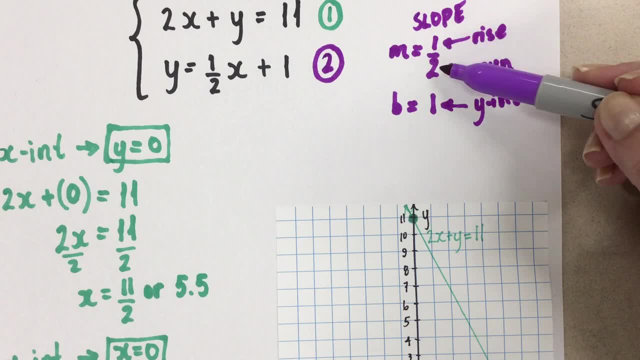 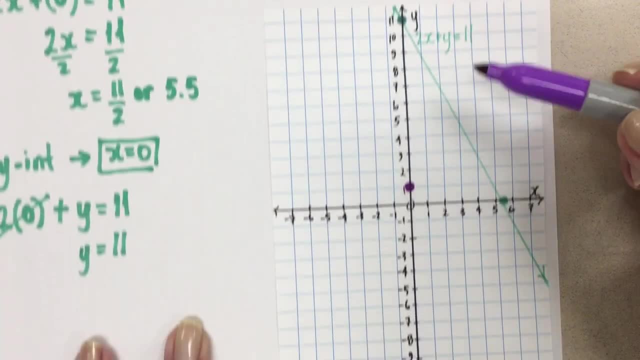 Now we're going up because this is positive 1, and we're going right because it's positive 2.. If there were a negative here, we'd be going down. We're going to go up 1 and right 2.. So from this point, we go up 1 and then right 2.. 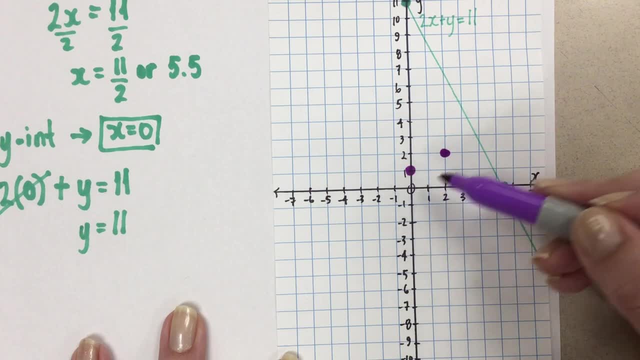 And right here is my next point. So there we have two points. That's enough to draw our line. If you felt comfortable, you could keep going Up 1, over 2,, up 1, over 2, up 1,, and so on. 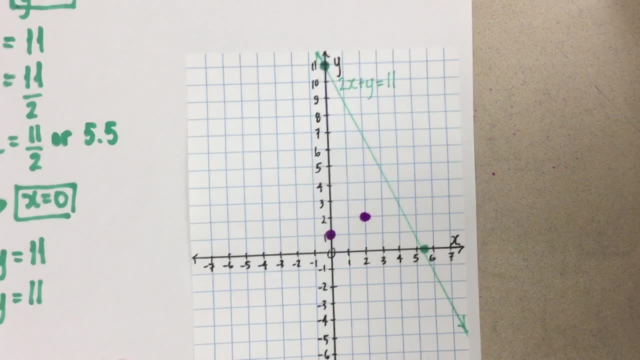 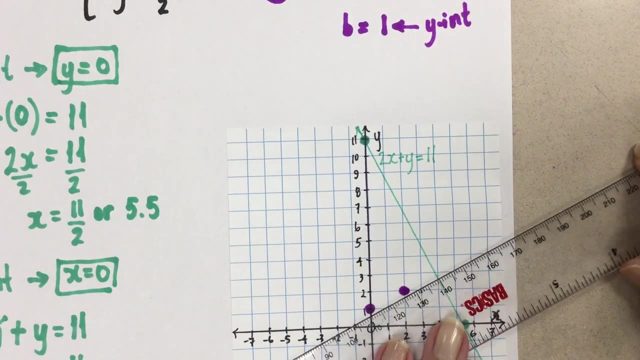 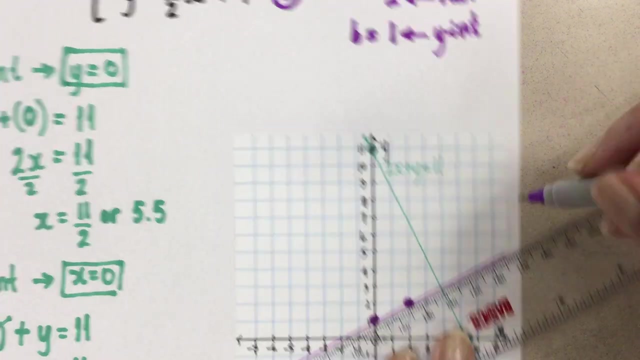 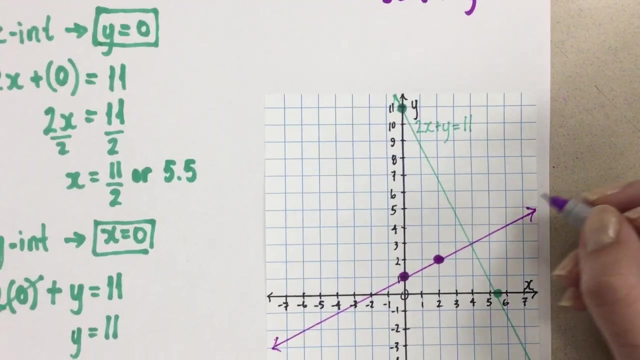 You see that you're forming that nice line with those steps. So now let's take those two points that we have and draw a line between them nicely with a ruler, And I will label this line also. Let's label it down here. 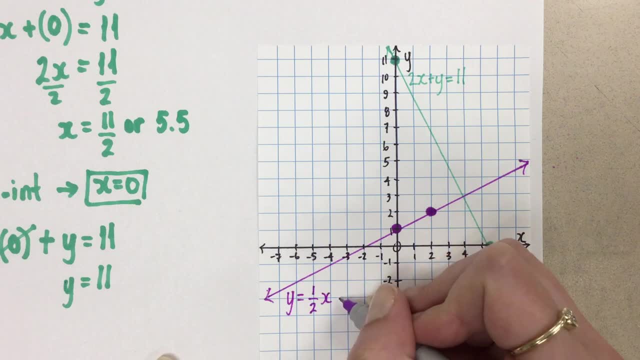 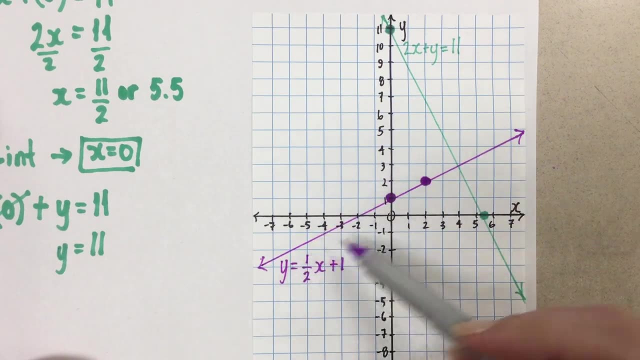 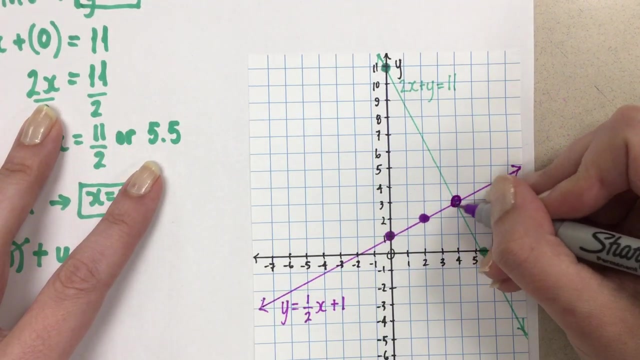 It was: y equals 1 over 2, x plus 1.. So here's my graph. The first line is here, the second line is here, and you see that they do in fact cross. They cross right around here. Now I'm drawing my point. nice and big. 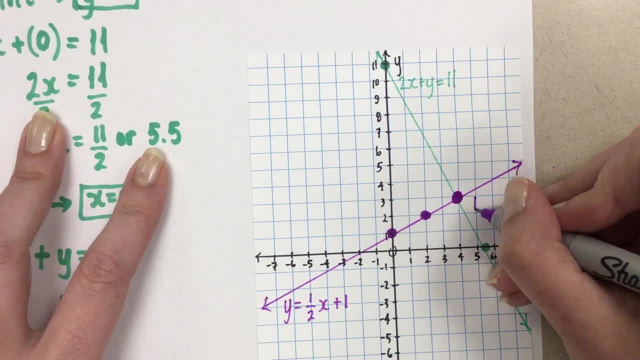 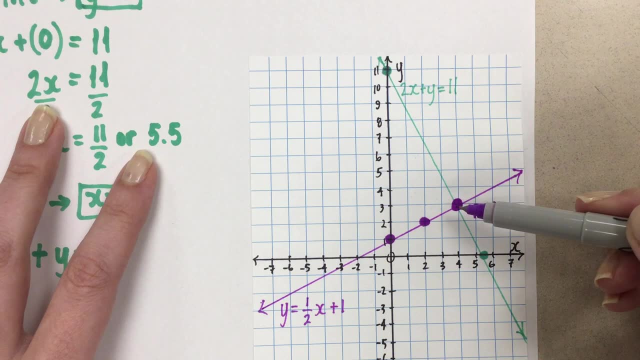 We call this the point of intersection. Sometimes we just use that acronym Point of intersection there. That is the solution to this system. Now you see how I'm a little bit off here, because we're graphing by hand and there's always a source of error when we're graphing by hand. 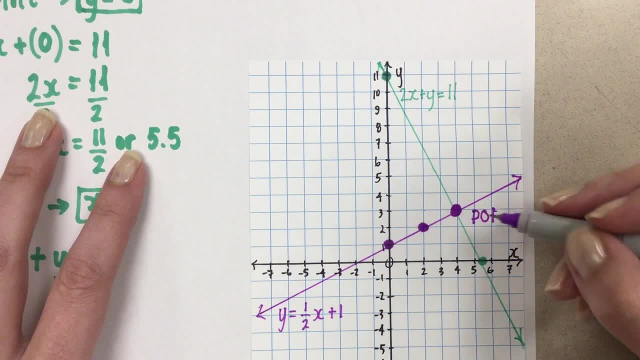 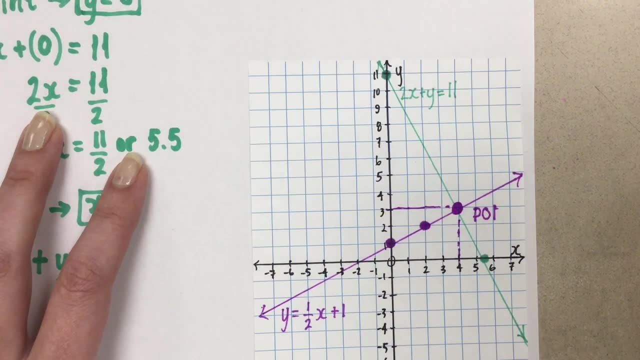 So you want to approximate that point as best as possible. In this case, to me it looks like the point is at 4. And 3 here. That's pretty close, So I'm going to go ahead and label that point. 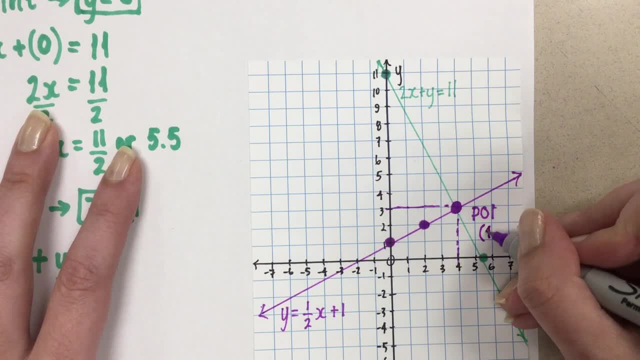 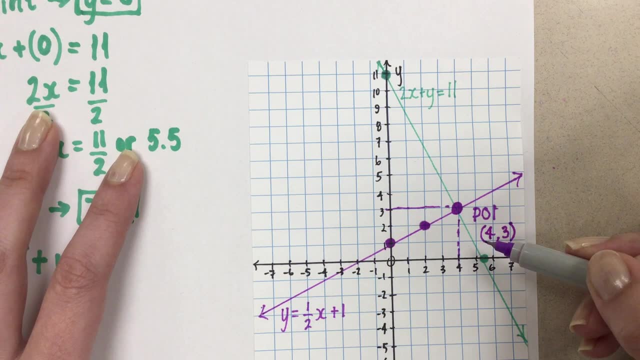 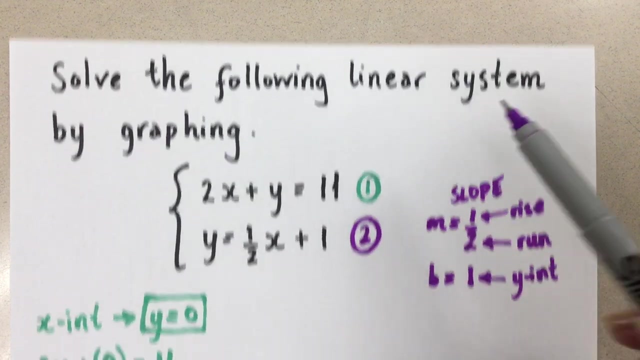 A point always has an x and a y coordinate. Remember x comes first and then y, just like the alphabet x, y. So our point of intersection is 4, 3.. When we're asked to find the solution or solve the linear system as we are here, 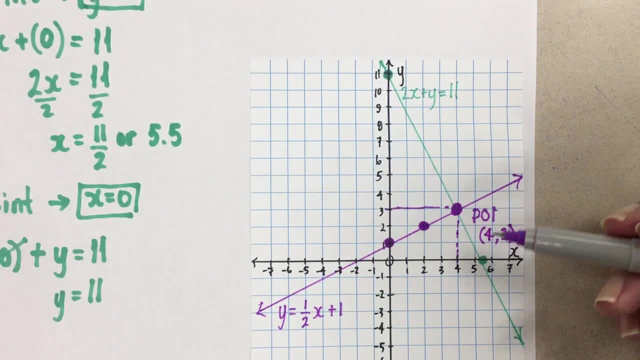 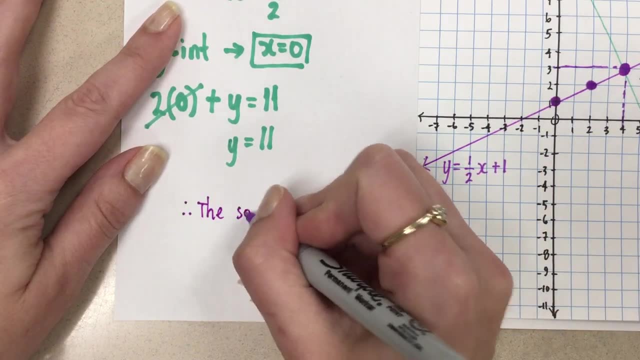 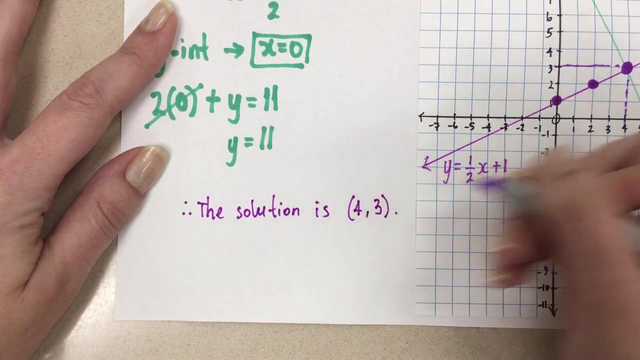 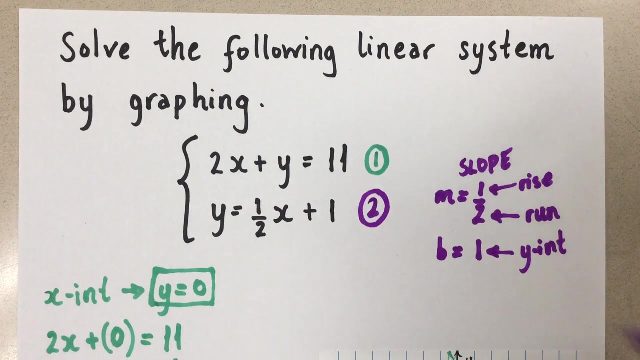 then that solution is the point of intersection. So here the solution is, Let's write this down: 4, 3. That's the point of intersection. So in this case our question just wanted us to solve for that point of intersection. 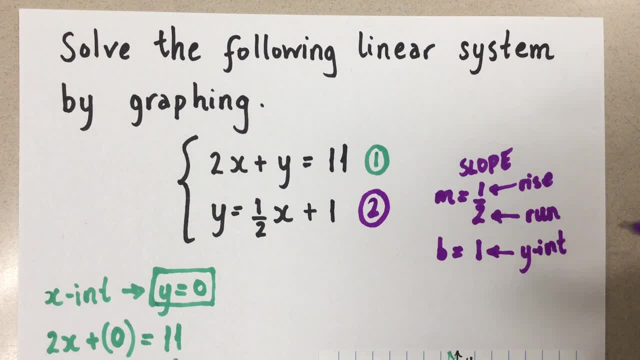 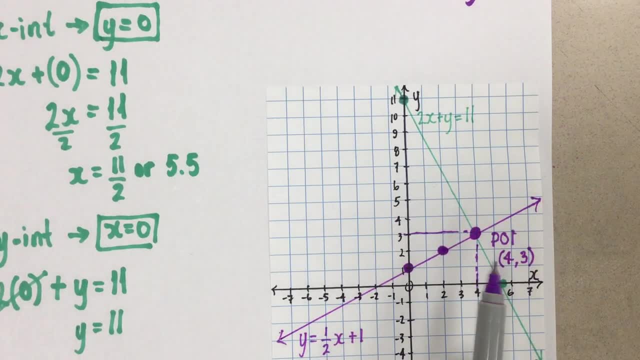 If we had some kind of applicable problem here with a realistic scenario, then we could describe this point of intersection further, because when we look at the point, the two lines have the same value at that point. Before the point, this line is below the teal line the entire time.